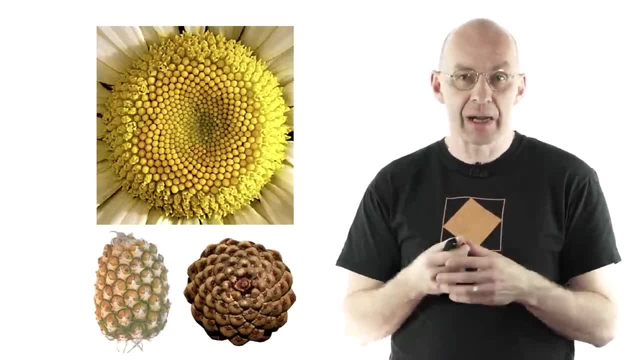 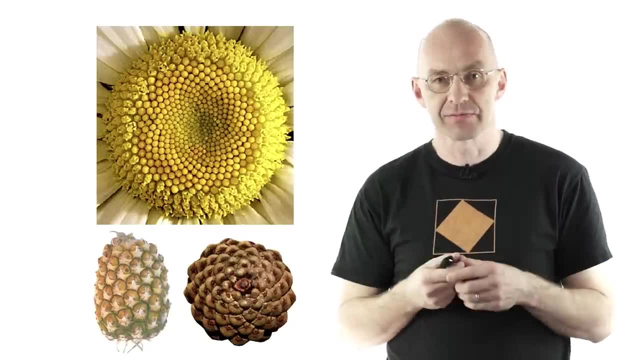 Well, for the past three weeks, I've been trying to come up with an explanation like this that really gets to the mathematical core that makes this happen, And I think I found it. So let me know how I went with this at the end of this. 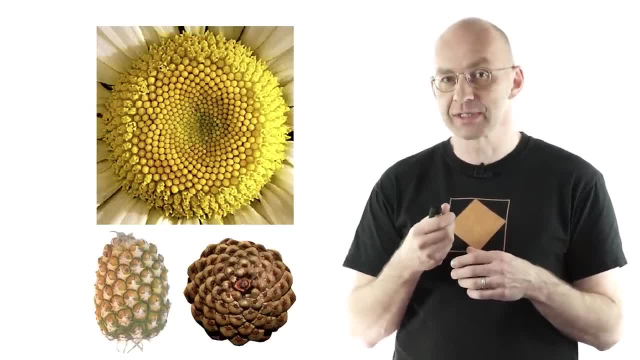 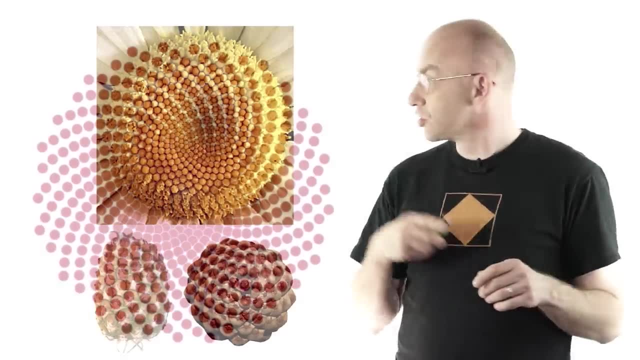 video. There's quite a bit more nice maths to all this that I'm going to talk about in this video. In particular, there's a nice connection with the golden ratio. For that, check out part 2.. So I'll focus on flower heads like this. 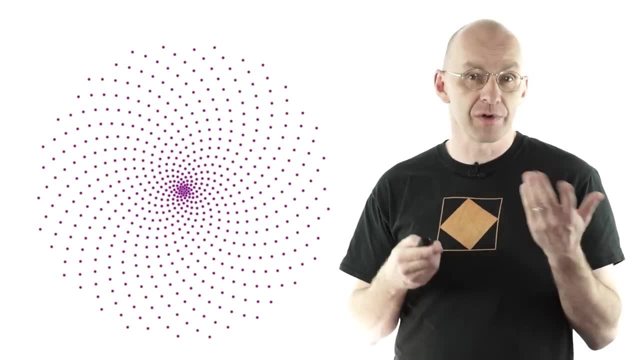 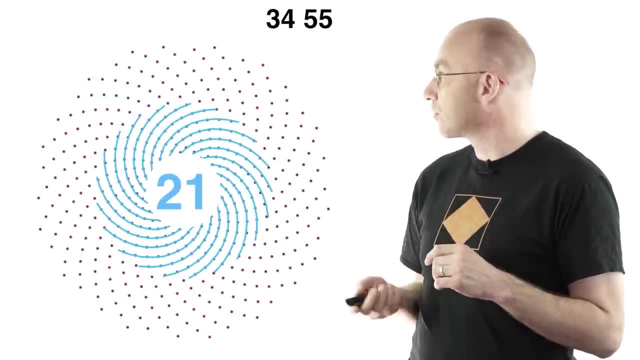 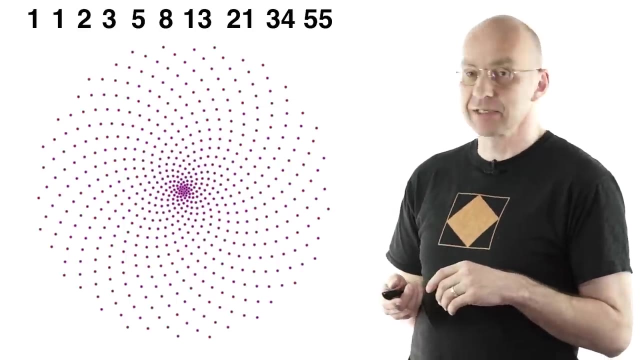 and let's have a close look. What jumps out at you are, of course, the spirals, So there's 55 going this way and 34 going the other way, and there's 21 if you focus in on the middle, and even further in there's 13.. And, of course, Fibonacci numbers. Now, before we 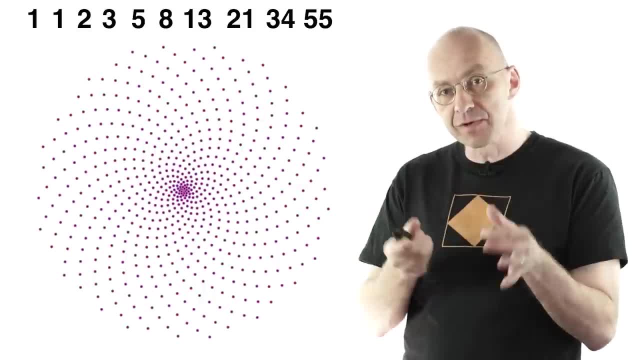 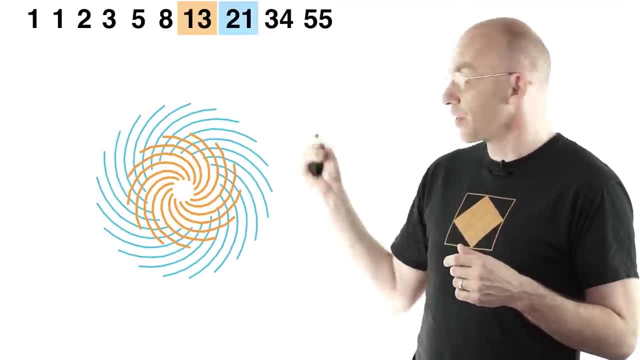 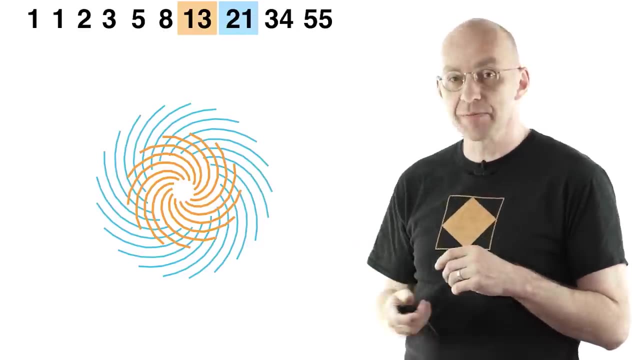 move on. I just want to emphasize that these different numbers are visible in different parts of the flower head, So the smaller the further in. So 13 is visible here, 21 further out, but there's always this region where they overlap. So consecutive numbers when you see them in the plant. 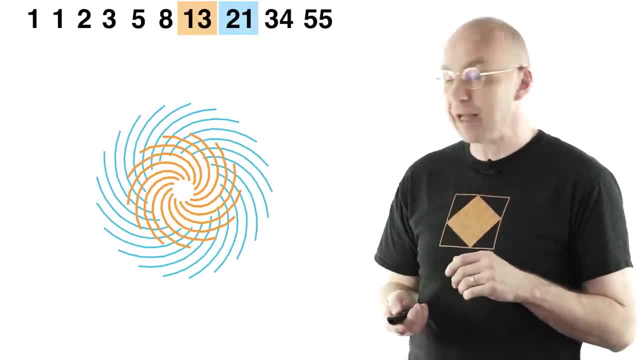 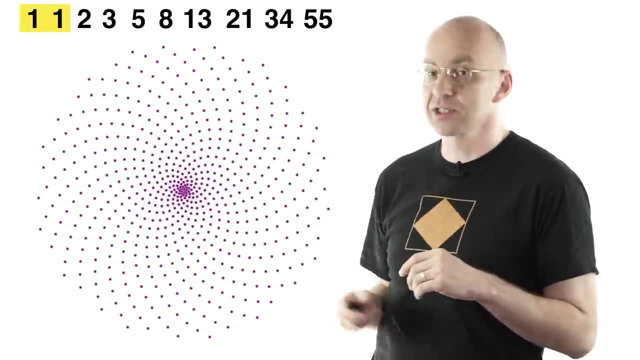 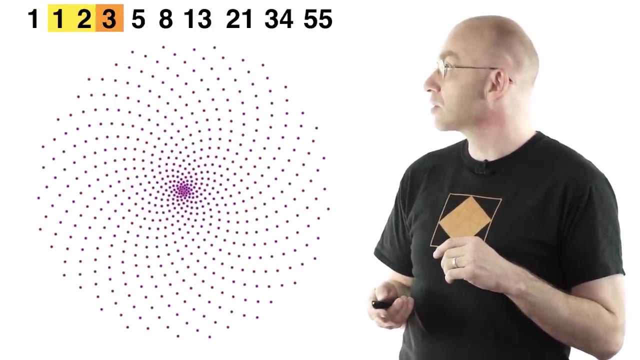 are occupying different regions, but they're always overlapping here with the next two, 21 and 34.. Now plants like this grow, so does the Fibonacci sequence, Starting with the two seeds, 1 and 1. we grow them like this: 1 plus 1 is 2,, 1 plus 2 is 3,. 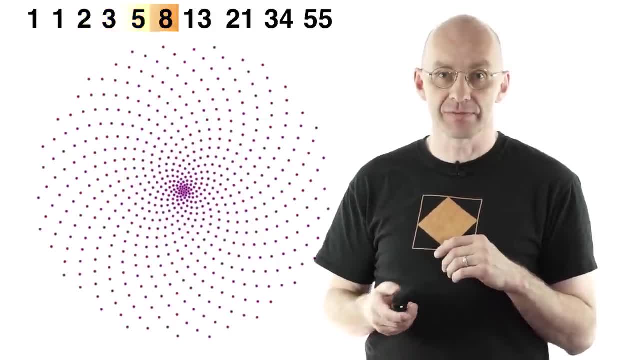 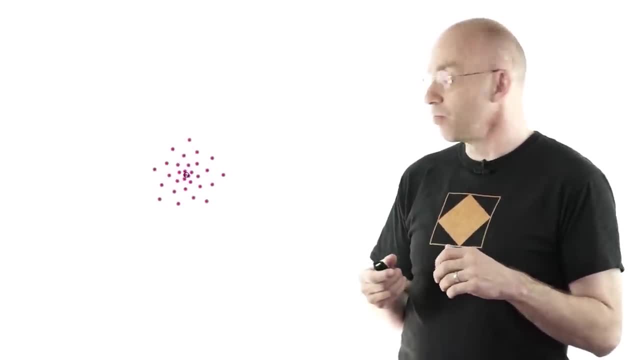 2 plus 3 is 5, 3 plus 5 is 8, and so on. Now, the plants that exhibit these spirals all have something in common: They all grow from a central point. So there's more and more of these butts. 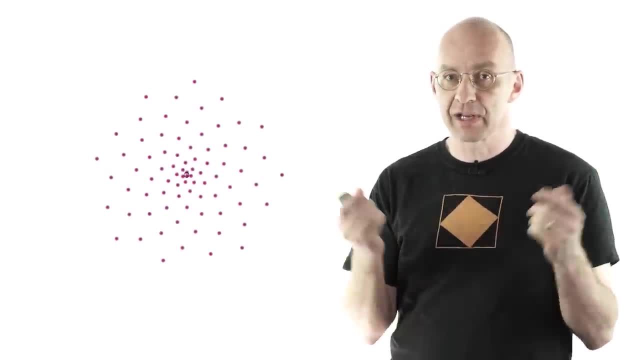 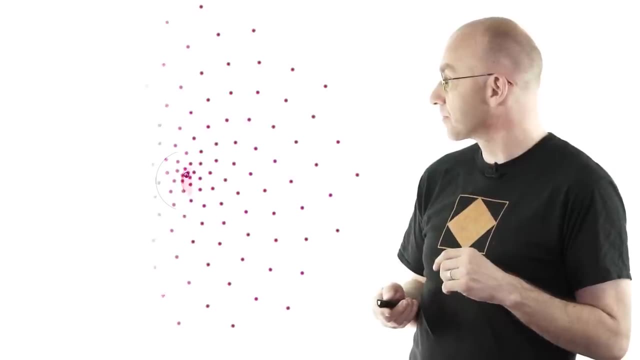 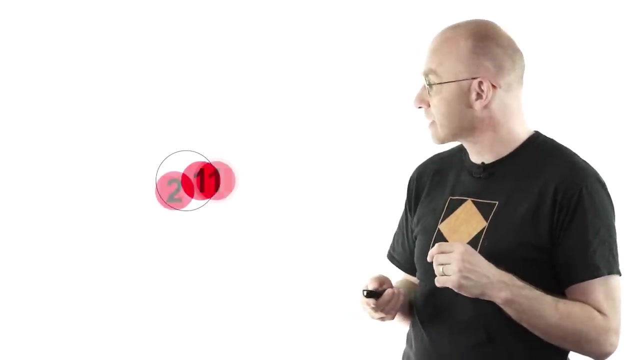 being pushed here in the middle and as they appear in the middle, they push everything out to the boundary and that gives this really nice homogeneous flower head in this case. So a bit of a more detailed look. So here we've got the first guy sitting, just sitting there waiting for the second one. The second one squeezes. 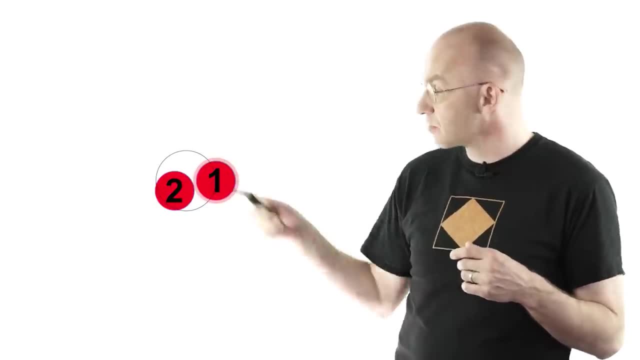 in like that. and then the third one has to kind of squeeze in above or below. There's a bit of asymmetry, so it goes for the top here and then, well, there's this gap here. that's where the next one is going to squeeze in. There's a gap. 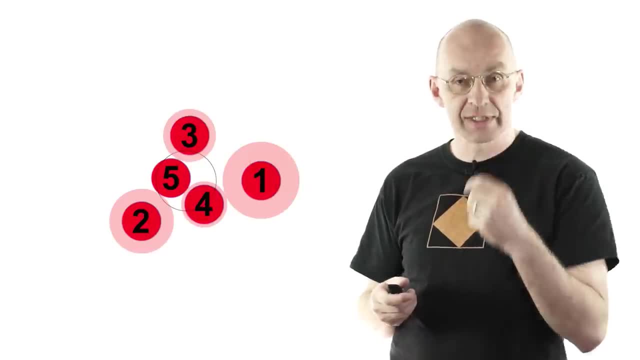 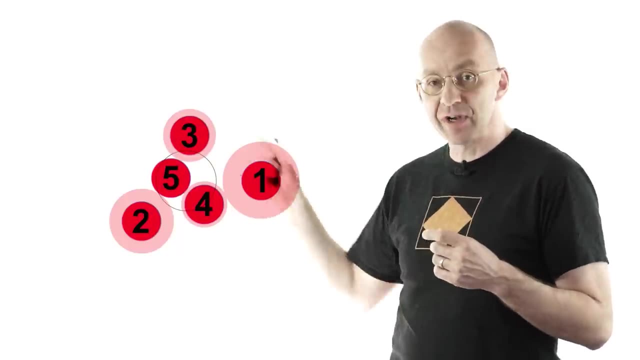 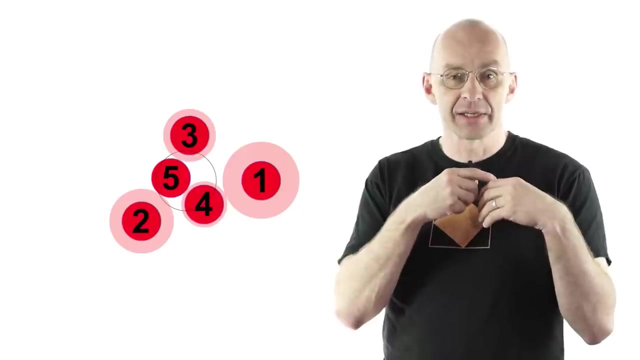 there where the next one is going to squeeze in. You can also see these seeds or butts are growing as they're being pushed out. So all this together establishes a very nice pattern, very, very quickly, very robust, and what that leads to is basically every seed or butt playing the same role inside the 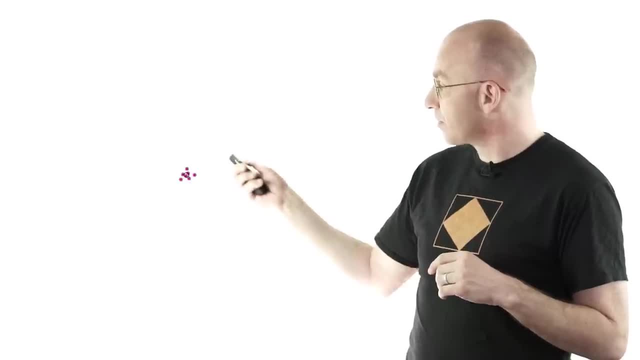 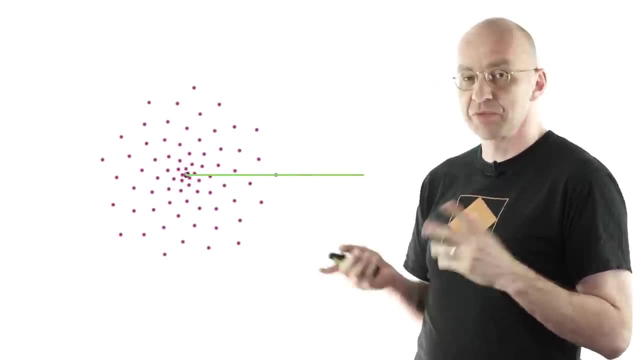 flower head. So some consequences of all this: When you have the plant growing, all the butts are being pushed out radially, so they actually move along pretty much straight lines. Another thing is, if you focus in on part of the flower head and take 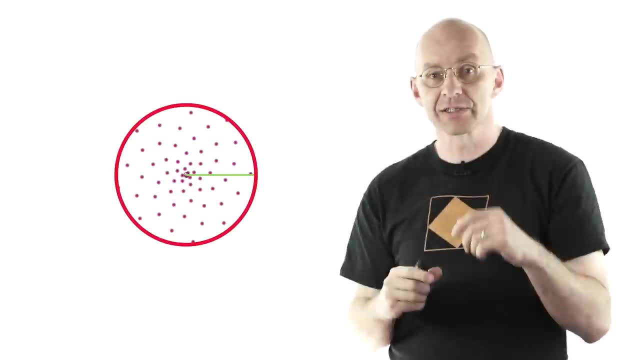 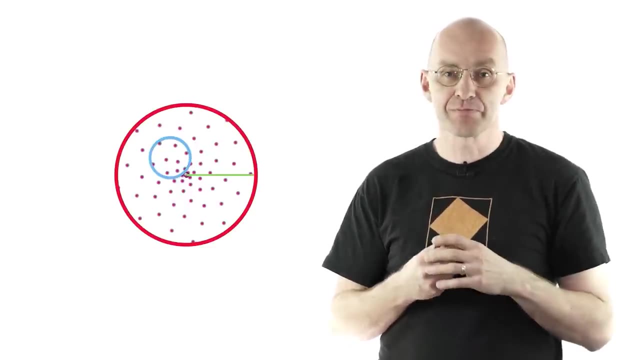 snapshots, you basically always see the same thing. You can kind of turn around like this: You always see the same thing. Then, when you have a close look again, you see that everything here is packed very, very densely, So things are being squeezed into the middle and everything is kind of 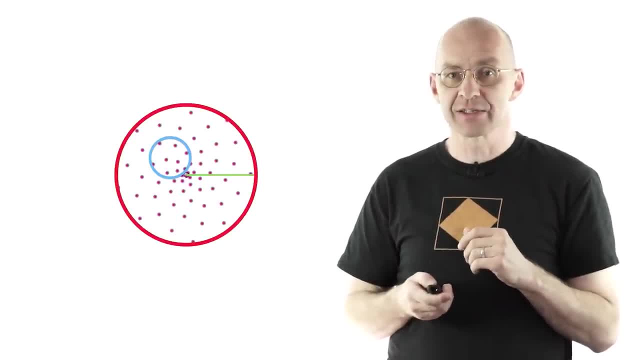 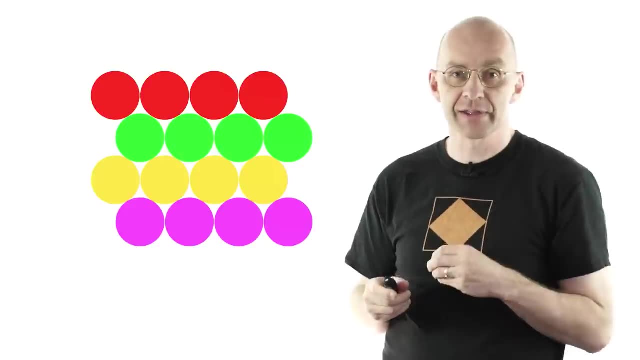 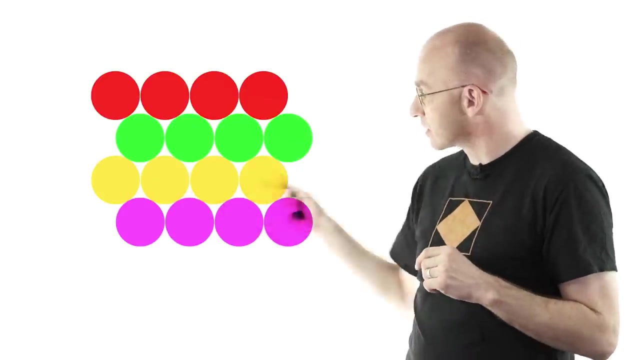 pushed out and you're really packing things as densely as you can. Now, if this was absolutely optimal- the densest packing of circle, like things like these, these butts, would really be this pattern here. You don't quite get there, but you get fairly close. So you've got these layers. 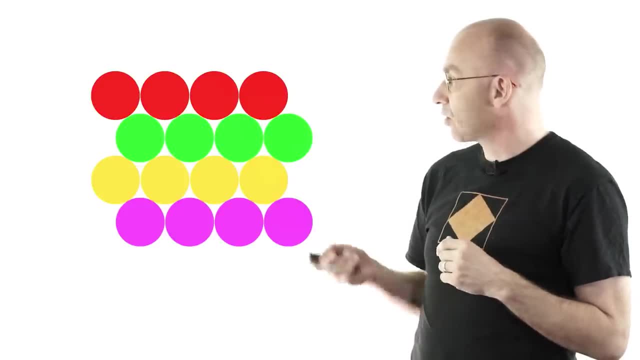 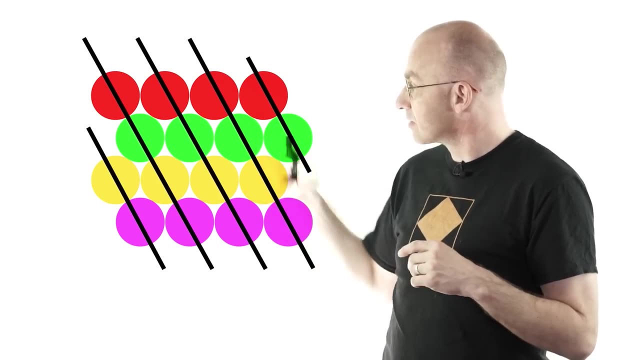 here and they're interleaving like this, and then you also get these circles aligning in certain ways and you've got another one going the other way. Now let's see where this sort of packing comes up in a real plant. There it is, You. 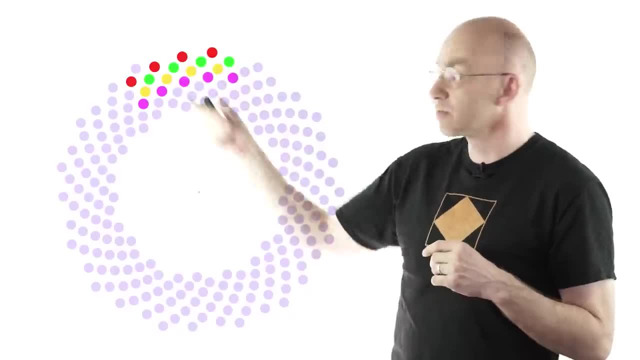 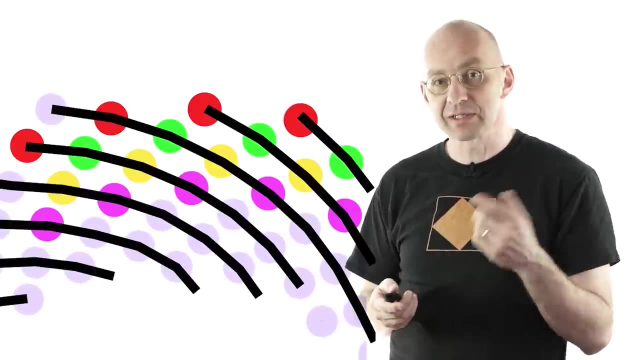 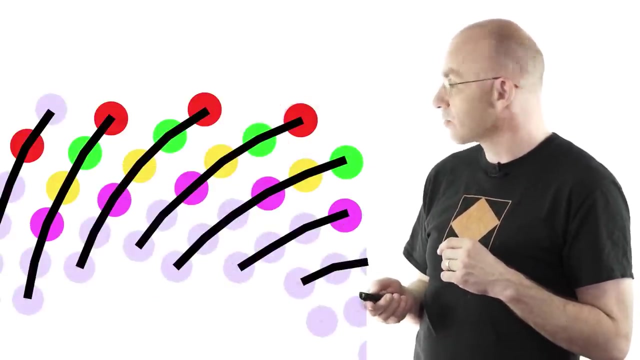 can pretty much take any part of the plant. you'll be able to fit this pattern in there. A closer look here Now we are two families. There's the first one, that's a family of spirals, now equally spaced, going around the center of the flower head, and there's a second one. 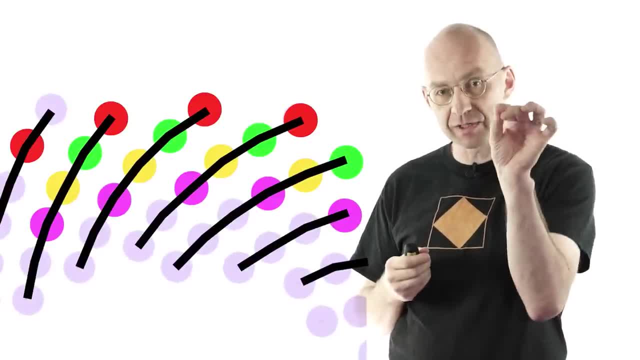 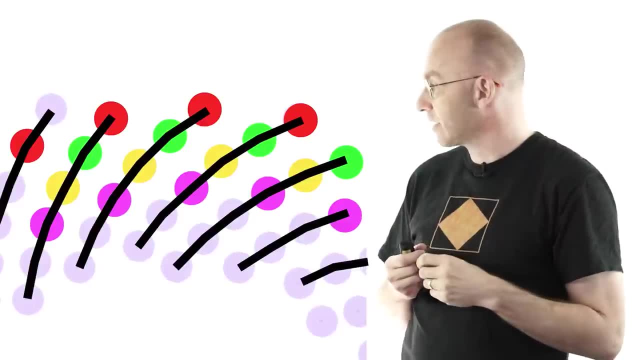 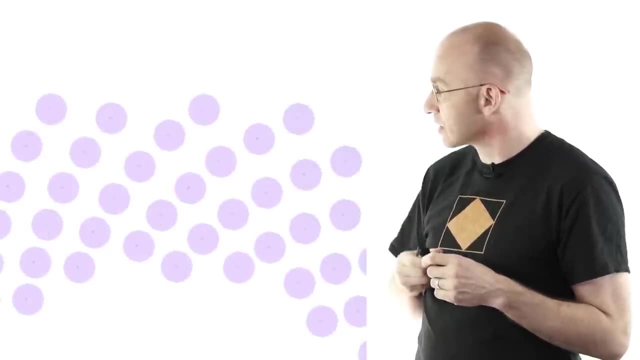 going the other way. It comes about very naturally just from this little stable pattern being established in the center of the flower and then everything being packed as close as you can. You get these two families of spirals happening. Now, if we focus in on this plant, we can actually see another. 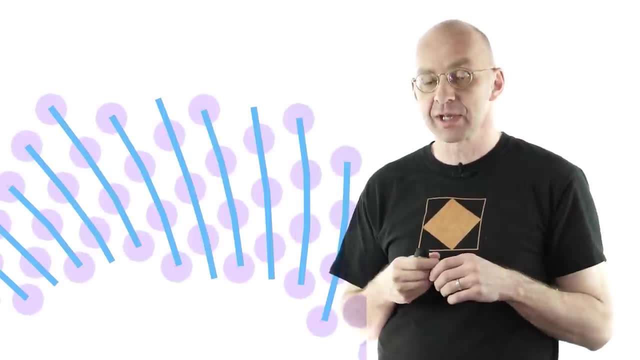 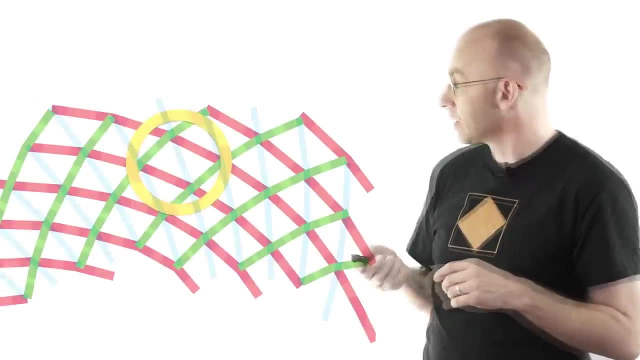 family of spirals. There it is. It doesn't jump out at you like the other two, but it's there and actually it does jump out if you extend them out further into this part of the plant up there. Let's have a close look. So the first two families of 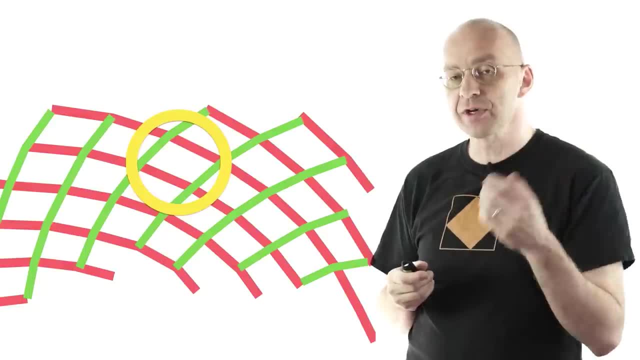 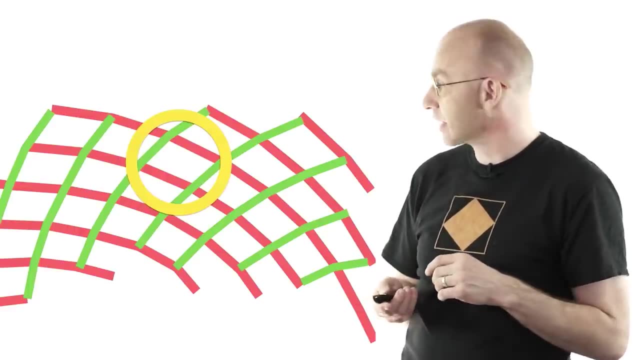 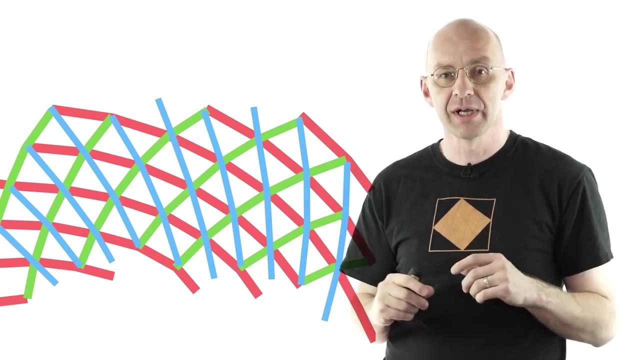 spirals. they make these diamond cells. and the third type of spiral, they form diagonals cutting through those diamonds. So I call them the diagonal spirals. And these three spirals being connected like this actually translate into the mathematical core that makes the Fibonacci numbers appear in flower heads like this: So what? 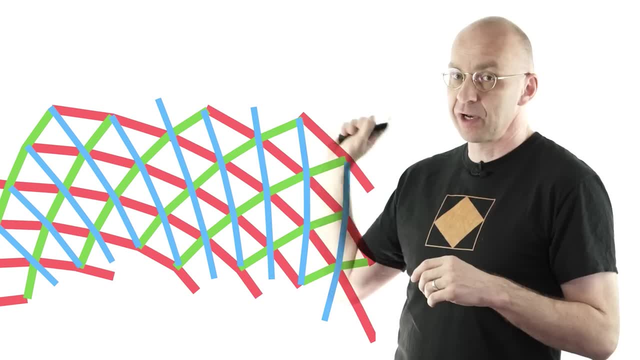 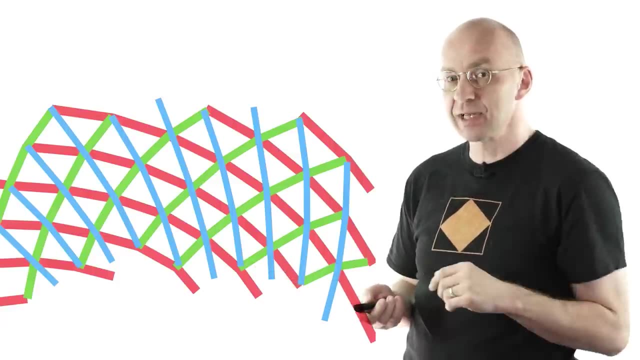 is it? Well, if you have a family of spirals twirling this way, equally spaced, like that, and another one twirling that way, equally spaced, and you look at the diagonal family like this and you count the number of spirals in these families, you always find that the number of green ones plus the number of red ones is 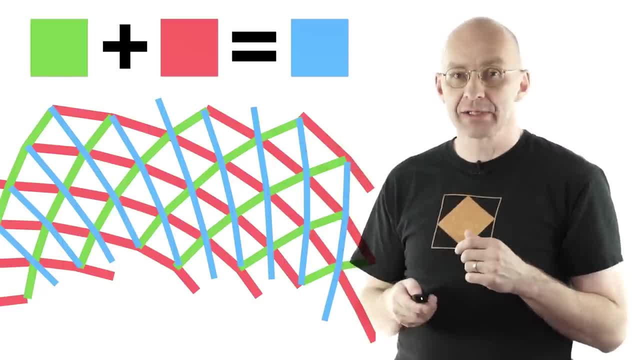 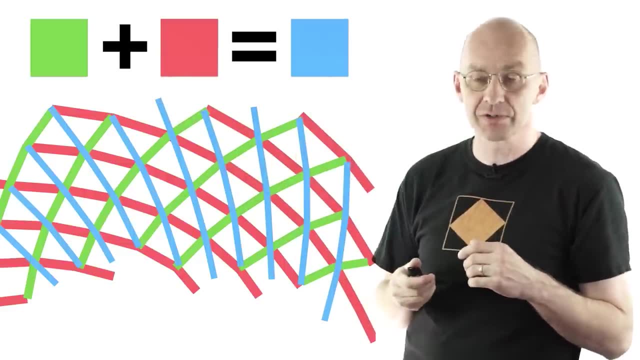 exactly equal to the number of blue ones, And you can already see the connection right. So there's two spirals, Two numbers, and they're being added up to give a third number, just like the way the Fibonacci sequence grows. I'm actually going to prove this to you at: 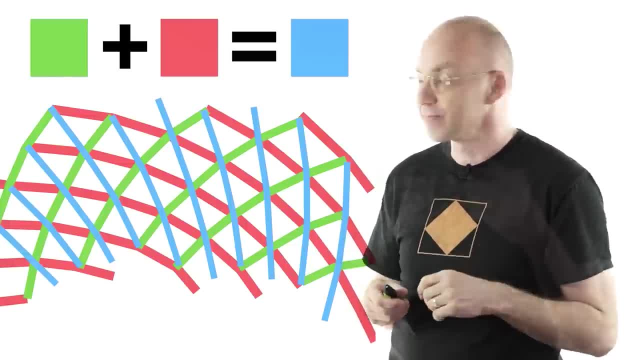 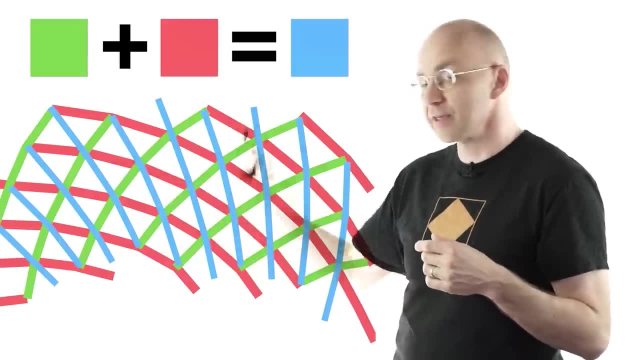 the end of this video. It's my own proof, very proud of it. So I have to do it, But let's just run with this. So we've got one number visible, that's the greens, and we've got another number visible, that's the reds. We don't have the blue ones yet. 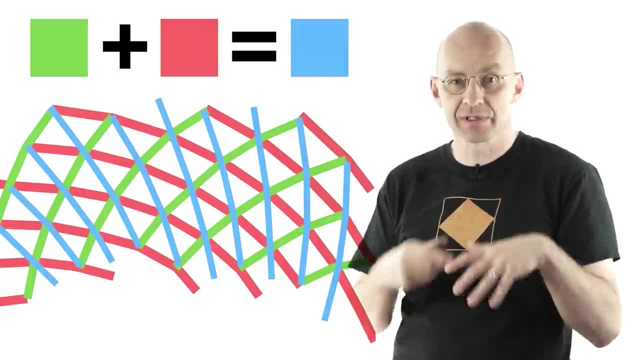 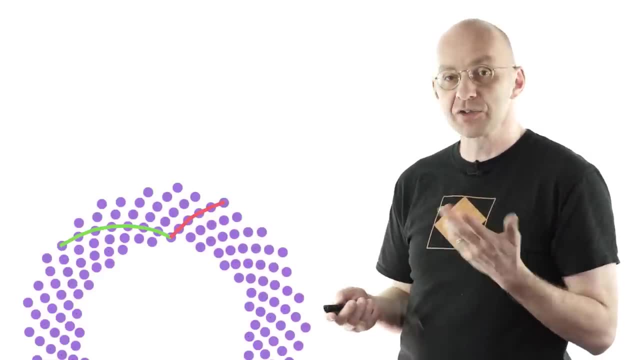 So how does the blue one come up as the next number in the sequence visually? Well, let's have a look here. I'll highlight one of the green spirals, I highlight one of the red spirals and I'll also draw in one of the green spirals. 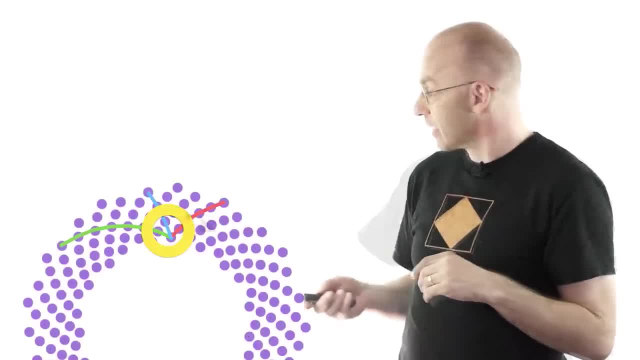 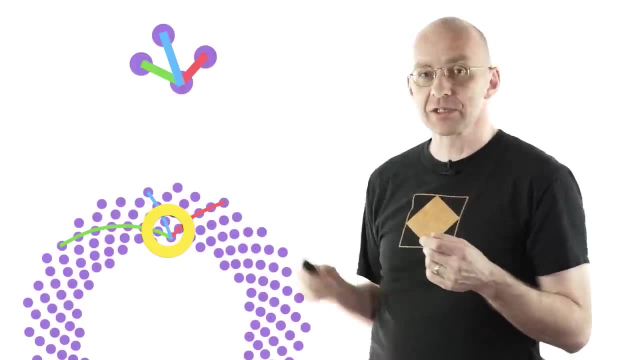 I'll also draw in one of the blue ones there. It's not jumping out at you yet. Focusing on this point magnified out over here Now, the spirals correspond to the shortest connections. I mean, the spirals are not there, you're just making. 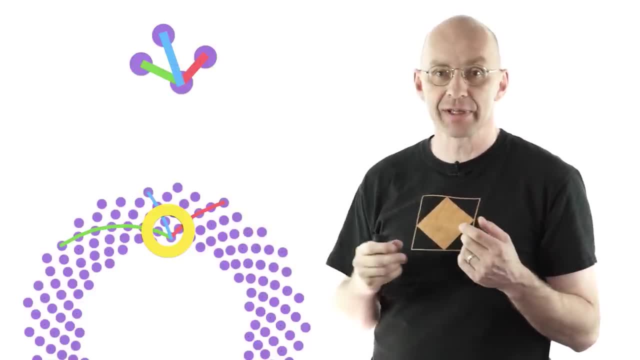 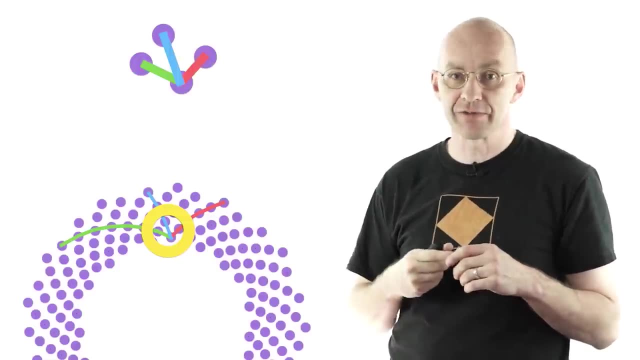 them up, basically, And what you do is you're looking for neighboring butts and then extrapolate these connections that you see here, And the neighboring butts here are indicated by the green and the red at the moment. So what happens when now everything gets pushed out further? Let's just go So you can see. 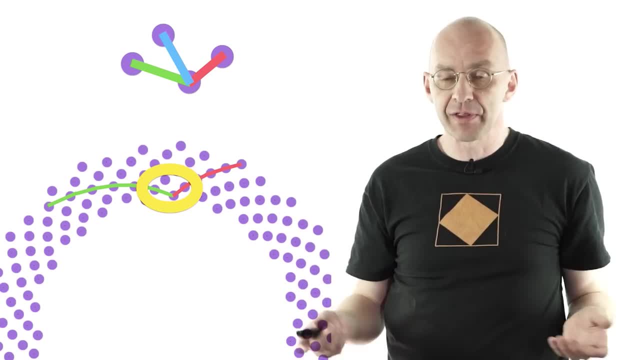 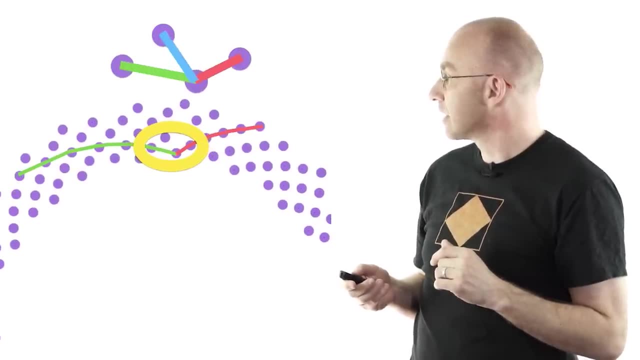 I mean, we've got the same arrangement all the way throughout, but everything kind of gets spread along larger and larger rings here, And what you can also see is that the length ratios change. In fact, this one has now become the longest connection and the other one are shorter, And when I take away the highlighting, 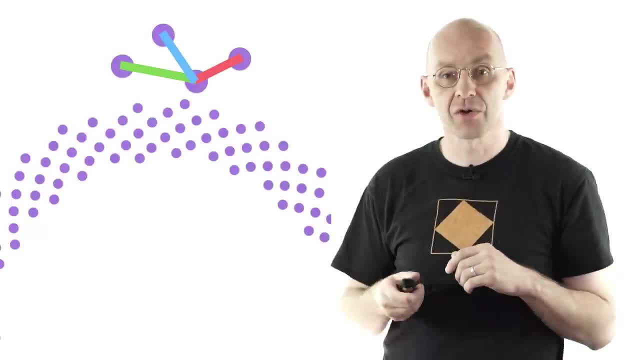 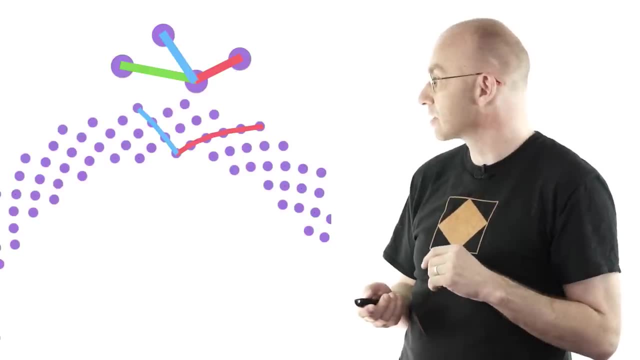 here and you close your eyes for a second and open them up again. you can actually no longer see the green, But what you can see now very clearly is the blue and the red. So that's how it goes. And well, we see the next type of spiral appearing there in the middle, and it 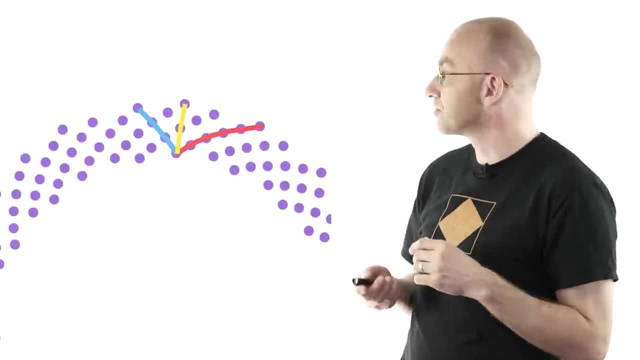 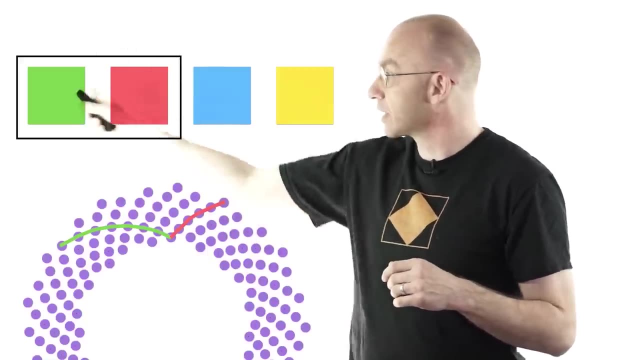 will become dominant further out as we push things further out. Okay, so we've had like four different kind of spirals here already, So we kind of start with those two. We know that the numbers here add up to the third number. These two are visible. This one becomes visible next. These two numbers add up to: 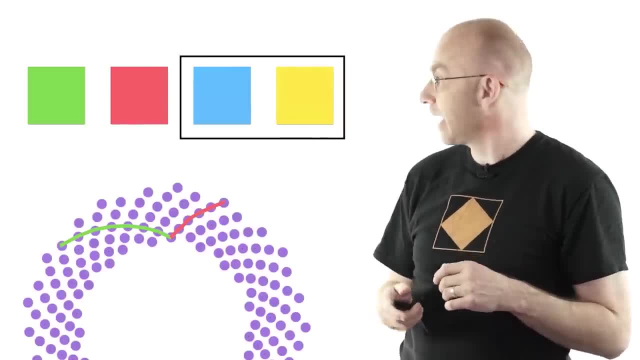 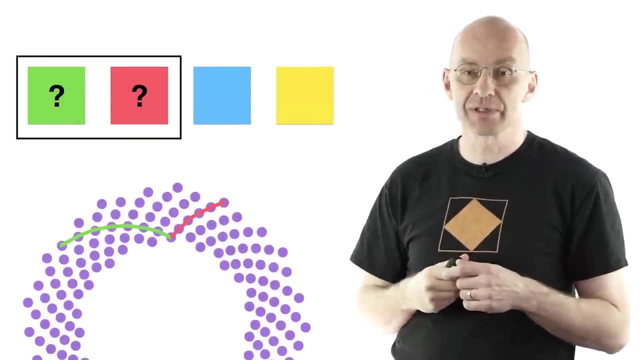 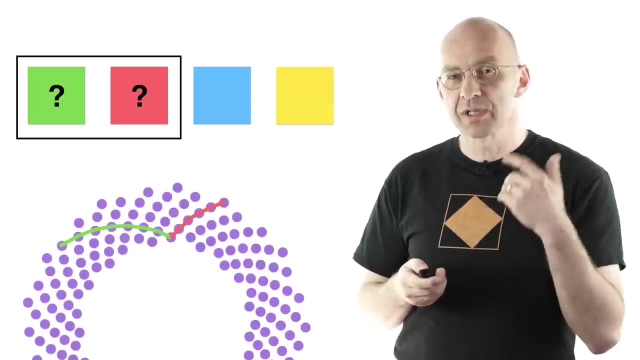 that one here- They're visible at the moment- That one's going to be visible next, and so on. So, starting with two seed numbers here, we get a Fibonacci-like sequence happening from that point onwards. Okay, so that's definitely part of the explanation. What it doesn't quite. 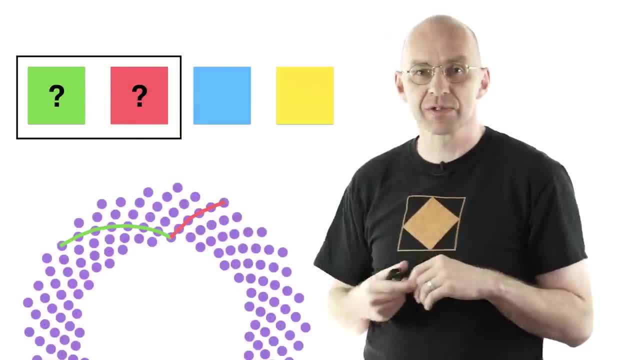 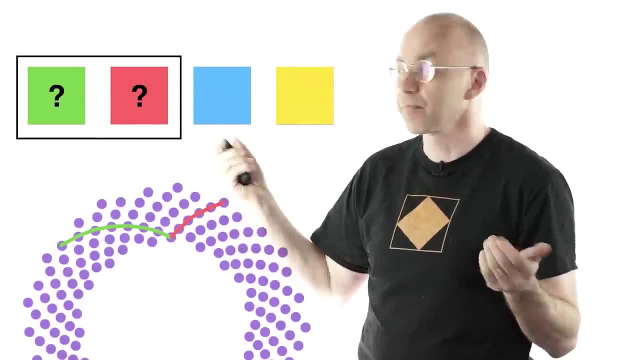 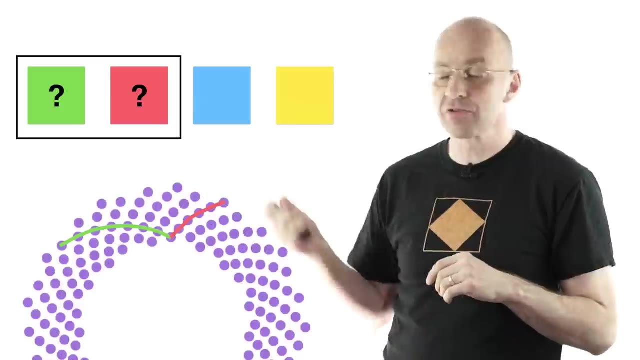 explain yet is: well, why do we start with Fibonacci seeds, like one and one and one and two and three or three and five and not some other numbers? Okay, could be some other numbers that pop up here first, and once they are established, everything else is determined by our rule. Well, there's a bit of confusion. 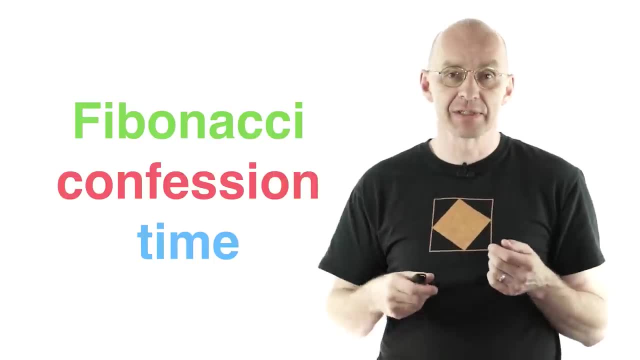 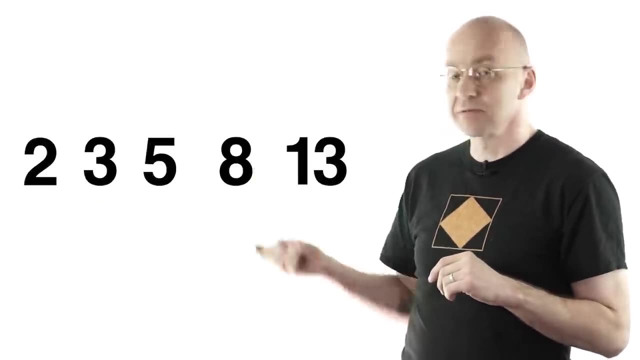 that I have to make. I mean, it's often claimed that the only numbers that come up in these plants are Fibonacci numbers, but that's actually not true at all. There's actually a lot of different sequences that come up, So there are the Fibonacci numbers here, but there are also, like double the Fibonacci numbers for. 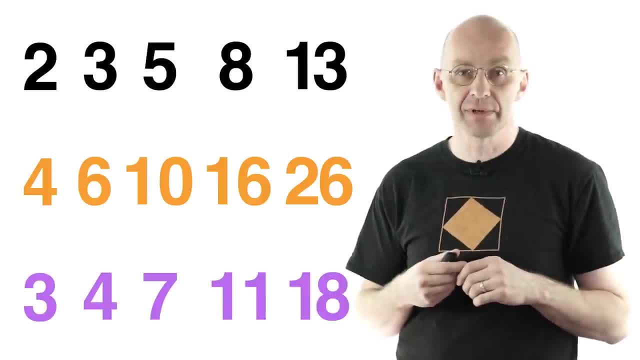 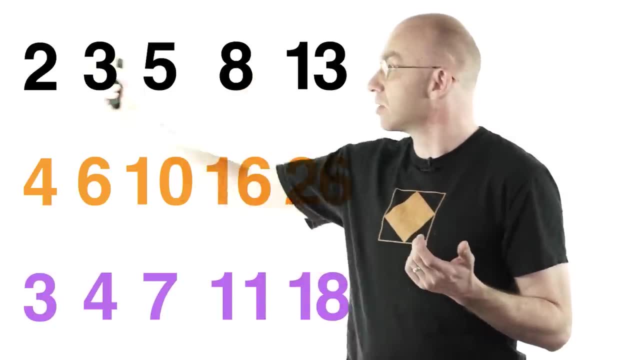 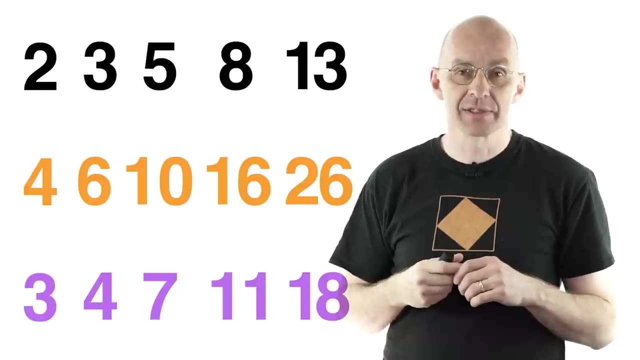 example, and there are also these guys here called Lucas numbers. So all these come up quite, quite a bit, but what they all have in common is that they follow our rule. So two numbers always add up to the next one in the sequence. Okay, well, there's still a bit of a predominance of the Fibonacci sequence. 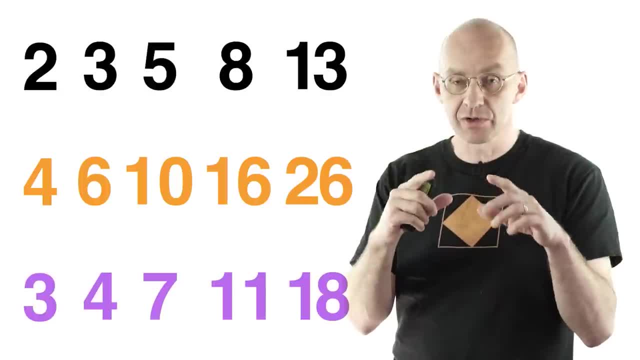 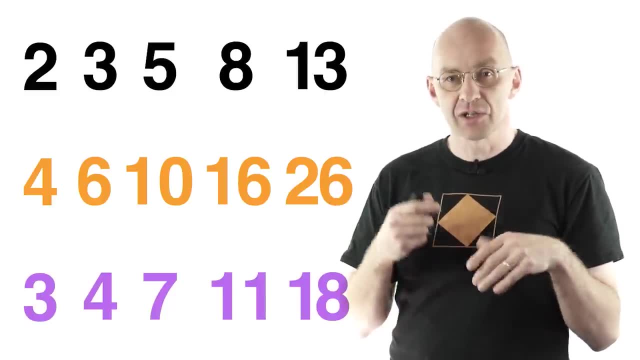 and how do you explain that? Well, you really have to have a close look at the individual plant and have to do a very detailed analysis there. and I'll link in a couple of papers in the description. It's a lot more complicated, it goes. 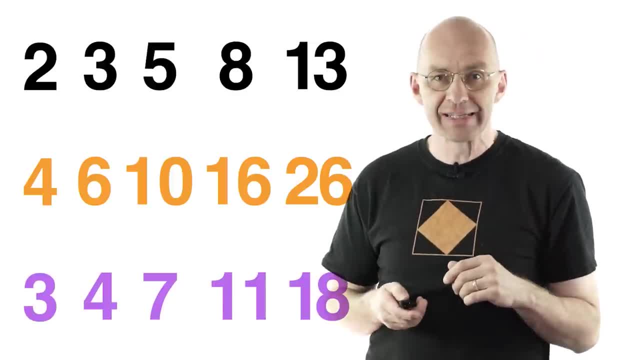 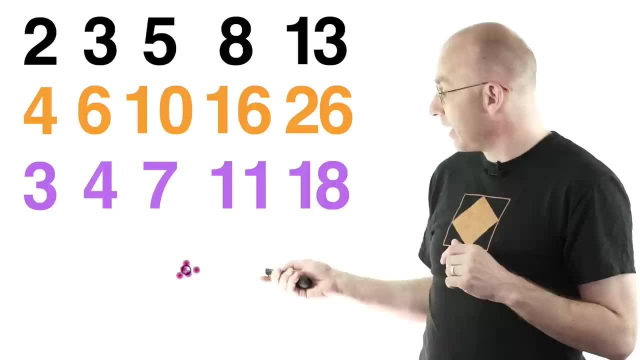 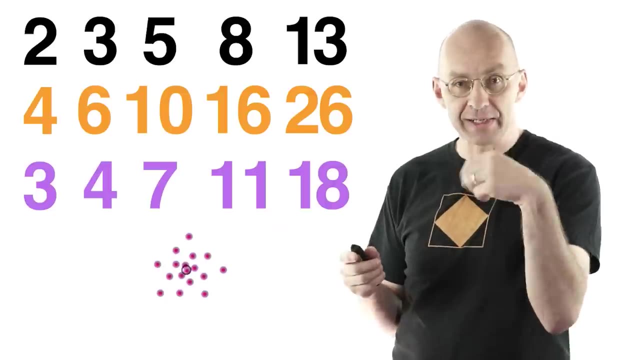 beyond what I'm going to explain here, I can just give you one more bit of insight into why you know these sorts of sequences should come up and nothing else. If you just think about it, a plant really also starts from very small numbers, right? It starts from one, one, two, three and so on. and since this pattern, 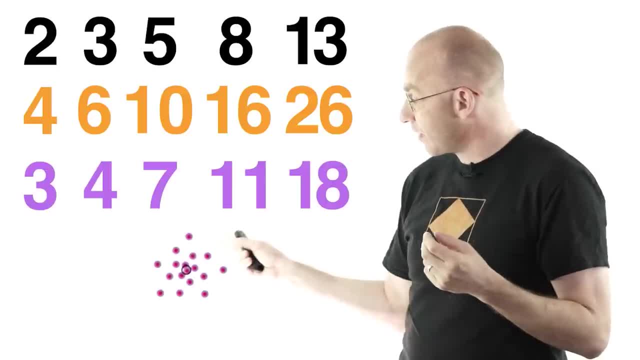 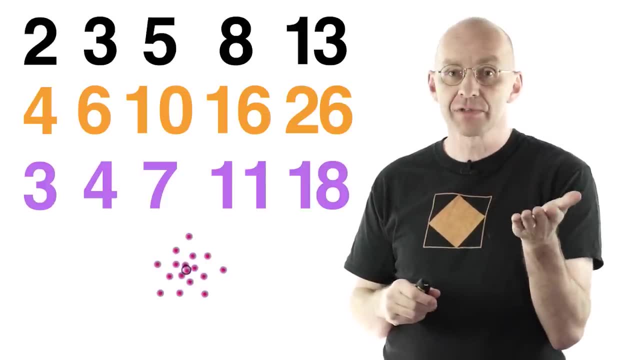 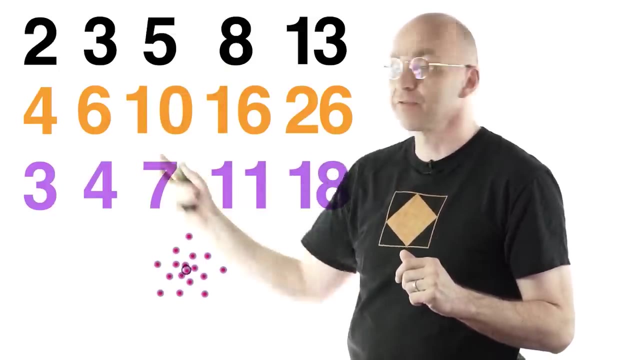 that I've been talking about is established very quickly. you'll also very quickly see like a ring in which two of these families are apparent. It's going to be small numbers of spirals in these families of spirals, right, And so it's going to be either 2 and 3 or 3, or 5, or 6 and 10, 4 and 6, one of those guys. 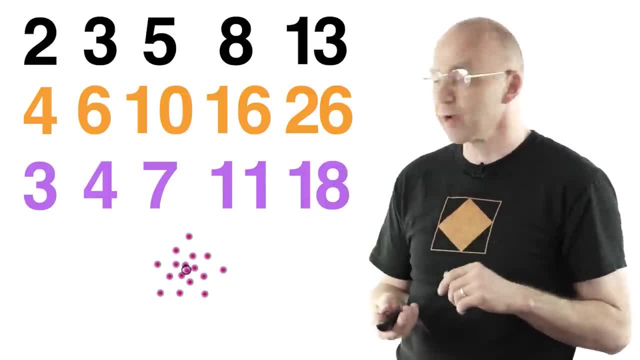 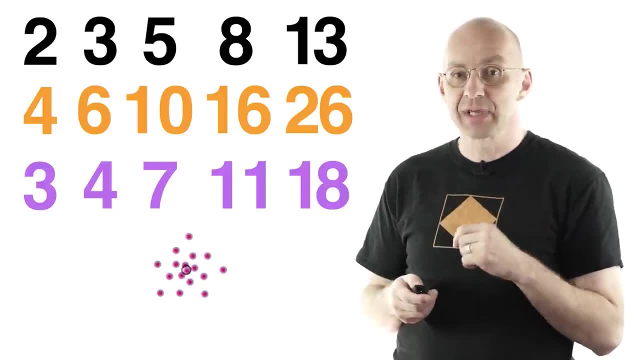 and it's going to take off from there. So you know it's quite plausible. Alright, so I'm quite happy with this explanation, so tell me whether you're happy too. Apart from that, I still want to give you my proof for why green plus red is equal to. 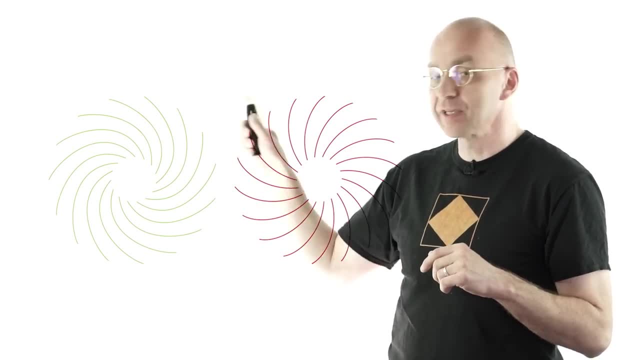 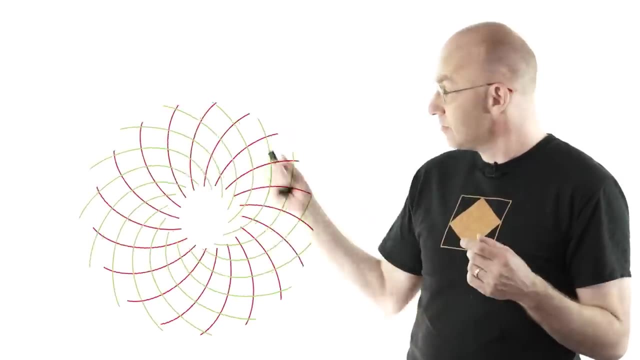 blue. So we start out with these two families of equally spaced spirals- and I've actually just made this up in a drawing program- and another one that kind of twirls. the other way, We overlap them like that and we draw in the family of. 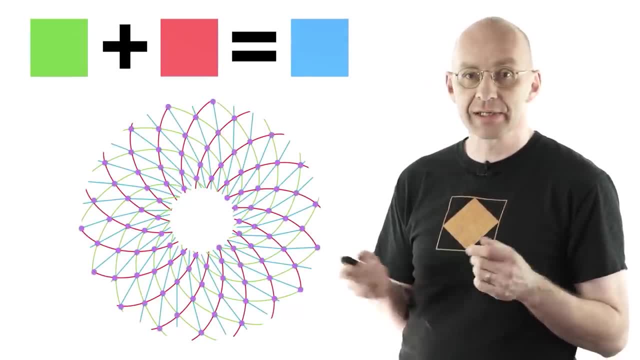 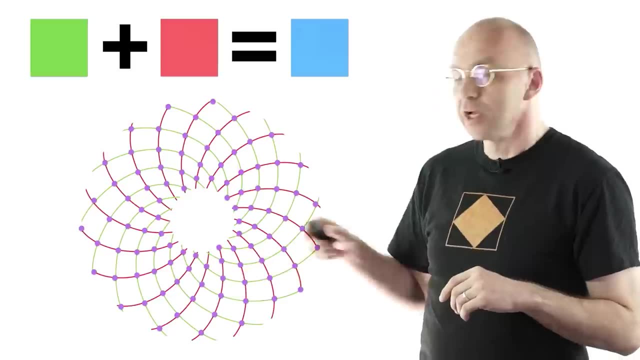 diagonal spirals. Now I claim that whenever we do something like this, doesn't matter how this comes about, we always get green plus red is equal to blue. Ok, so here's my proof. So we circumnavigate this ring and we start at this corner, and first we follow one of the red spirals and we can't go any. 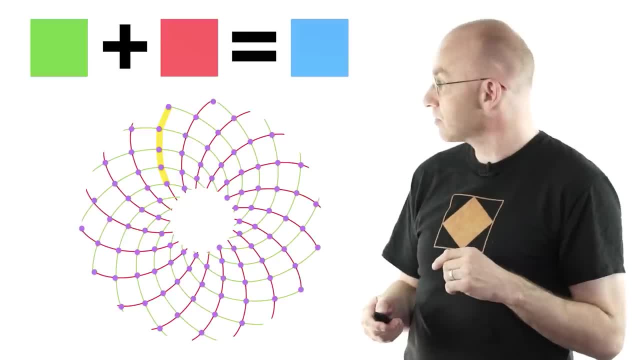 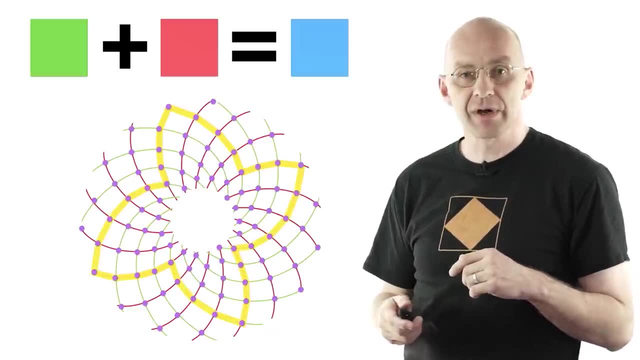 further. Then we switch to one of the green spirals, follow that one for a while, then we switch to a red one again, and then to a green one. red one, green one. It doesn't really matter how you do it exactly. it doesn't matter as long as you. 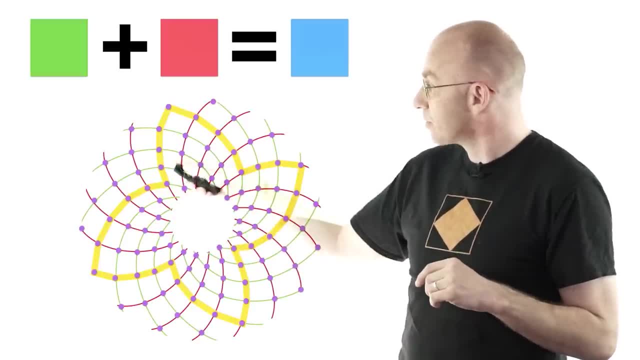 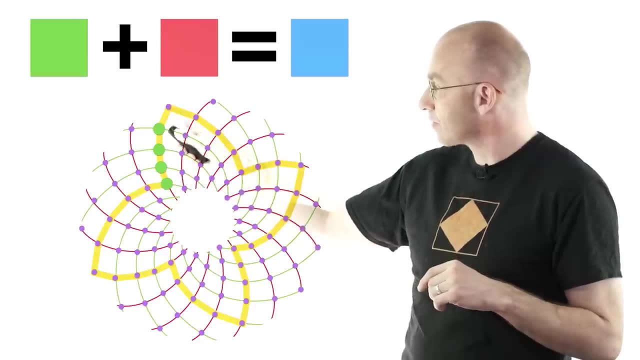 make a closed path like this yellow path. Now the points of intersection here on the yellow path we highlight. So first make those all green, so green from this corner on up to there. then in this corner here we put red and we go up to. 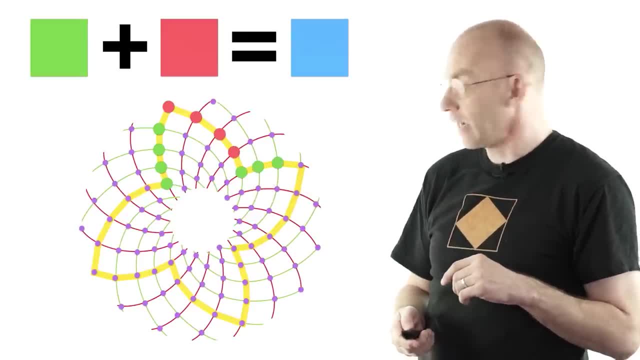 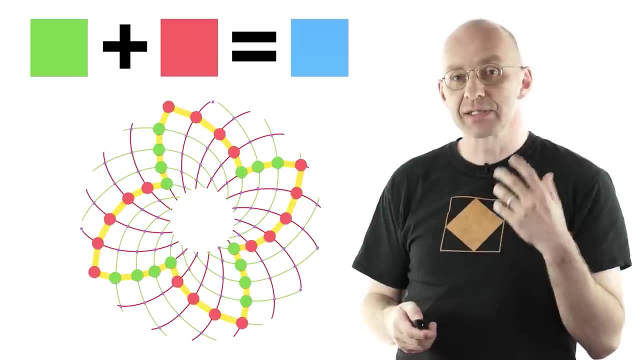 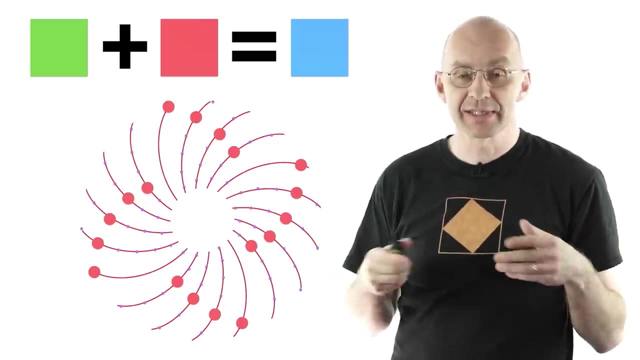 here with red and then again switch to green and then keep on going like this all the way around. Alright, and now you can actually see at a glance that green plus red is equal to blue. Here we go. Every red point is exactly one red spiral. It means there's exactly as. 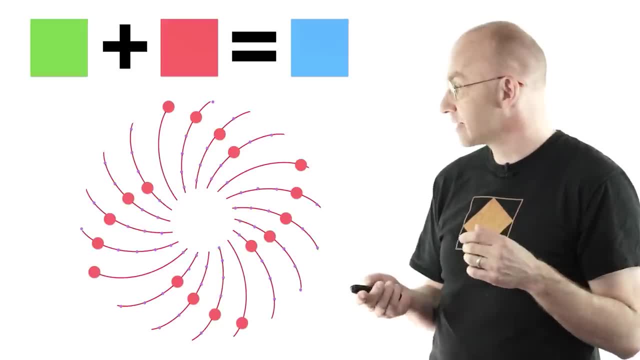 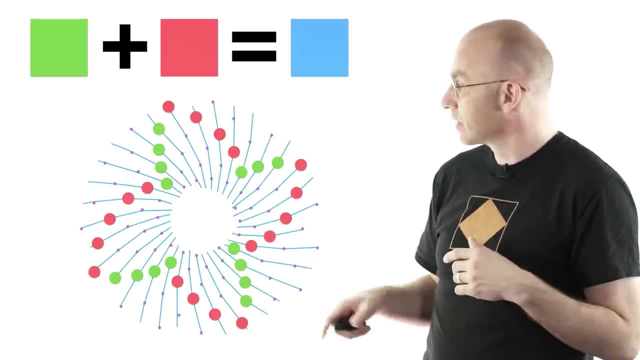 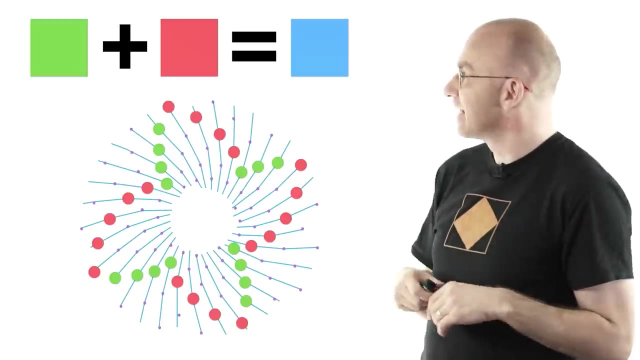 many red spirals as a red point, And the same way there's exactly as many green points as the green spirals. On the other hand, there's exactly as many points as there are blue spirals, and that shows at a glance that green plus red is blue.